control of your network, which device can authenticate to your network, which device can authorize within your network? Because when you implement a NAC solution, when you implement NAC solution, you have to implement policies. You have to implement policies, You have to define. what kind of controls do you want to? 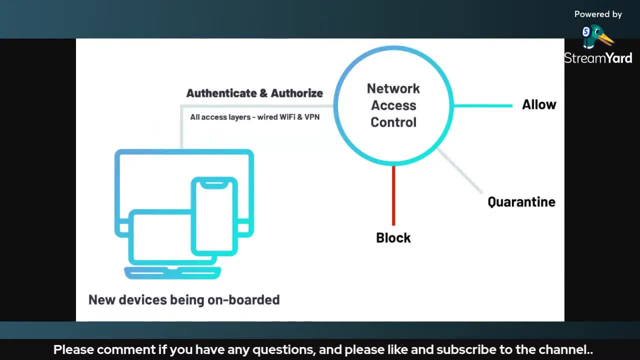 have in place? For example, do you want to have antivirus solution in place for any device to connect to the network? Do you want to have the latest security patches for any device to connect to the network? What are the different policies that you want to have for any endpoint? 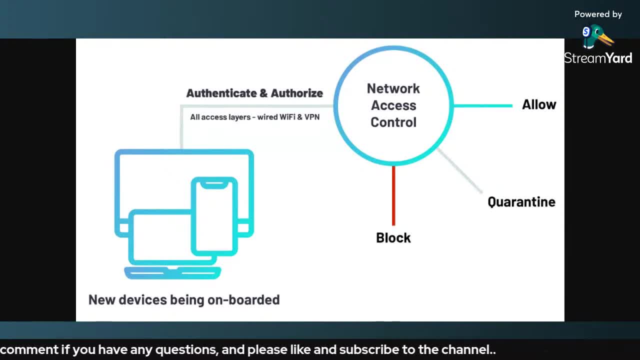 device to be connected to your network so that user can access your network. What is the importance of having a NAC solution these days? Because these days there are a lot of devices. So without a NAC solution, if anybody connects to your environment, you 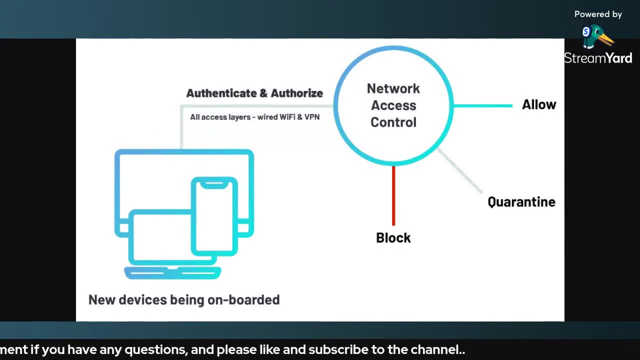 know it is harmful to your environment, guys, because if there is no proper antivirus solution, if there is no proper patching to the endpoint, you can imagine yourself what can happen to the network. Okay, so here, what you basically do is, when you implement a NAC solution, is you implement. 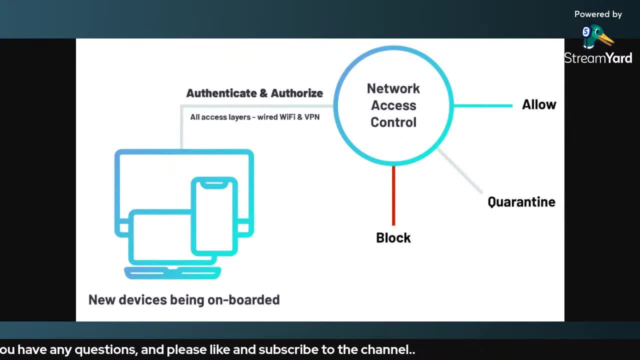 a baseline security. So you define a baseline state. you mentioned by defining a policy so that you allow, which type of devices you will grant, which devices you will block, which devices you will- you know quarantine. So these are the three you know resultants of having a network access. 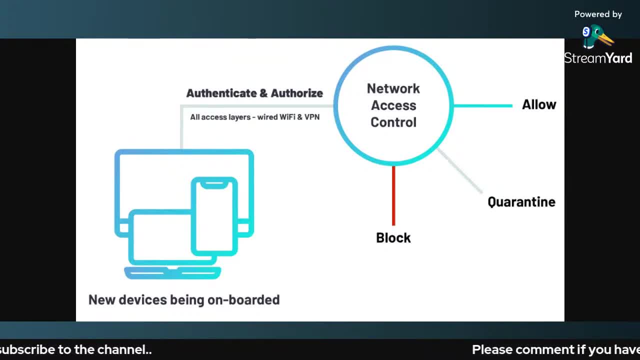 control in place. Okay, so, whenever, as discussed in this diagram, any new device comes on board, you authenticate it, you authorize it And, accordingly, you take these three steps. So here you have a NAC solution. Okay, so these are the three steps. So, when you implement, 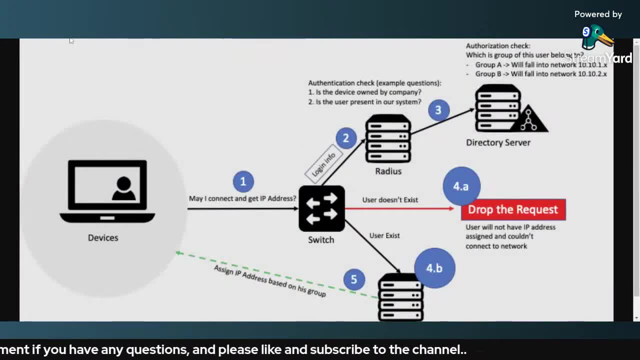 three actions. now let us see how these steps actually happen, one by one. okay, so let's say there is a new device on the network, so the new device joins to the network. it asks for an ip address. that is the first thing that any device would do for okay, so it asks for a ip address. 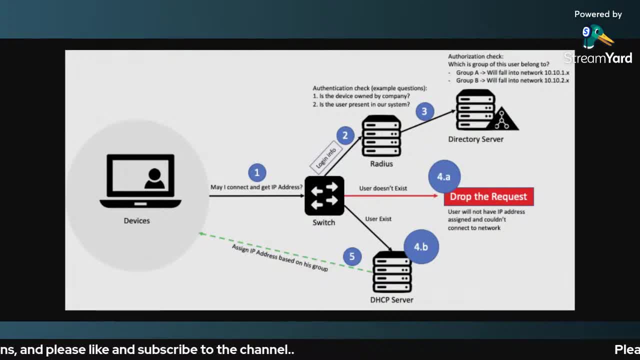 so where will it get the ip address? from the dhcp server. but not so quickly in case of a solution. the switch actually passes the device information on to a radius server. remote authentication dial in user service is the name of the radius server. so what a switch does is